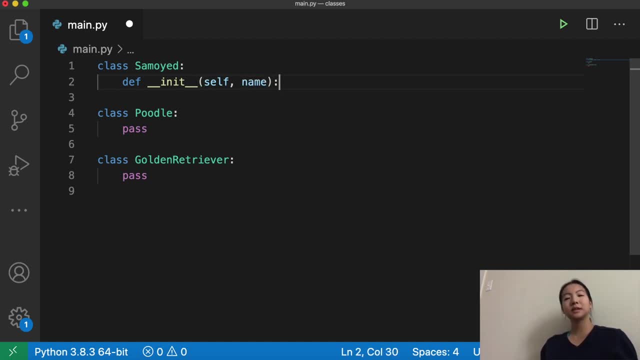 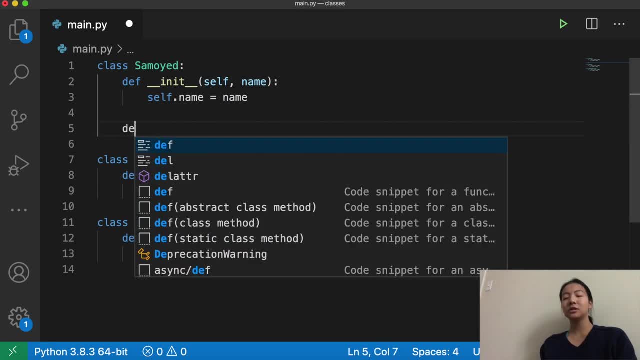 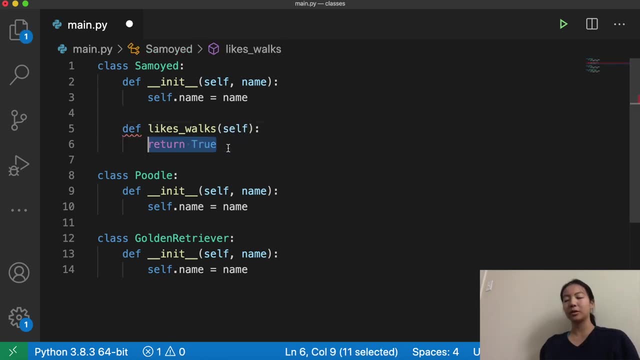 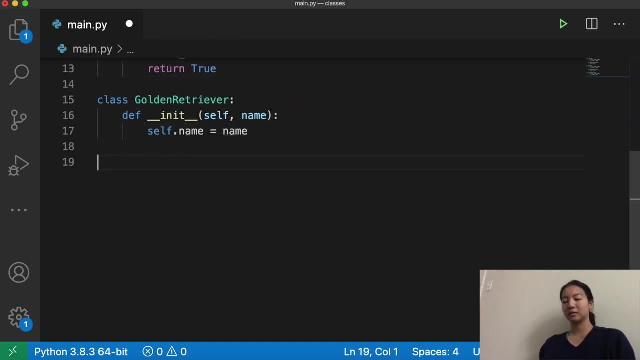 function literally copy and pasted three times. In addition, if we had another function like likes walks- And of course all of our dog goes like walkos, So we are going to paste these everywhere. So what we're seeing here is a lot of code repetition, because 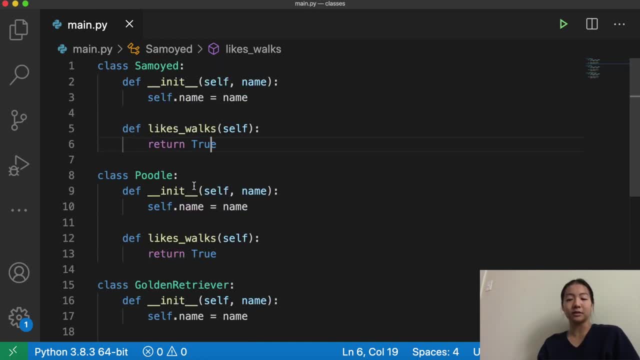 these two functions are basically copy and pasted for all three of these dogs if we take a step back and we think about this in real life, while Samoyed poodles and golden retrievers, they're all a breed of dog. So what we can do in. 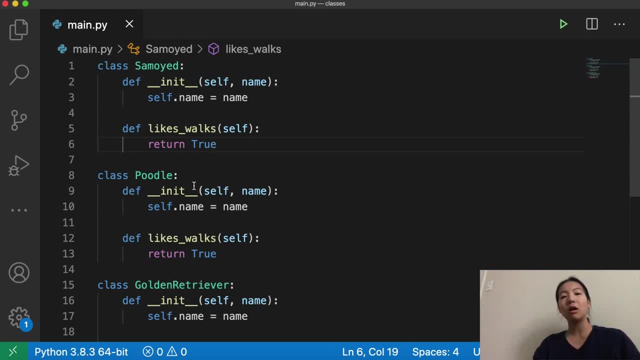 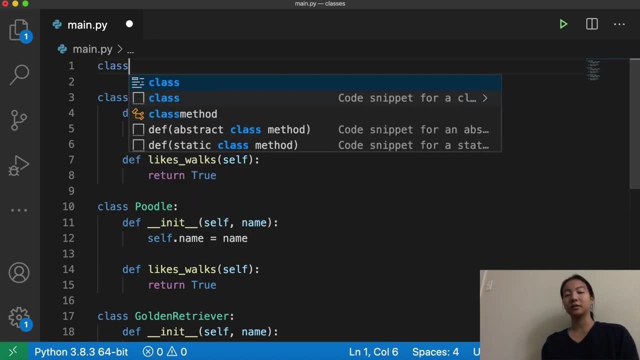 Python is. we can actually add a parent class to all these classes which unifies them as that type of object. we can create a superclass called dog which basically would have all the properties and functions of a dog to share among all the breeds. So here we can say a knit and then we can give it. 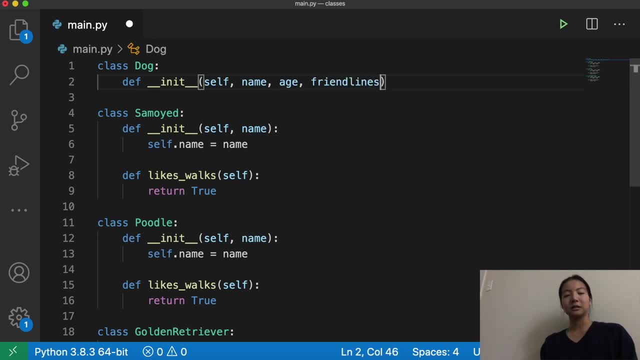 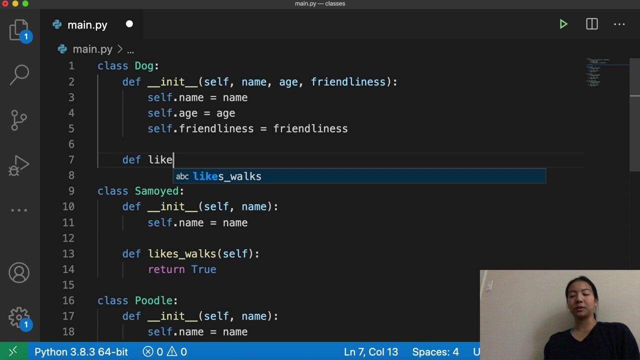 even other things like age, friendliness, etc. And here let's do: self dot name equals name, self dot age. we're just initializing all of these attributes within our class. all the dog was like the walk. oh, so we're doing likes walks self. And this is true, Okay, so now. 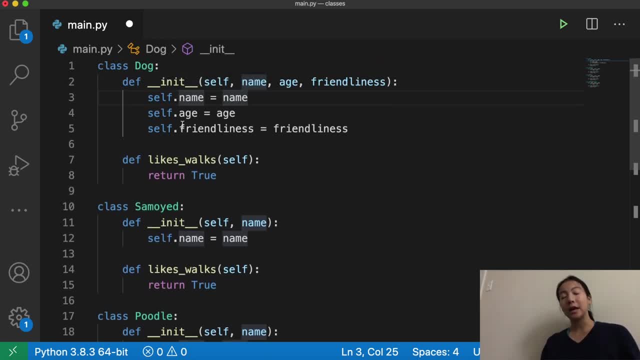 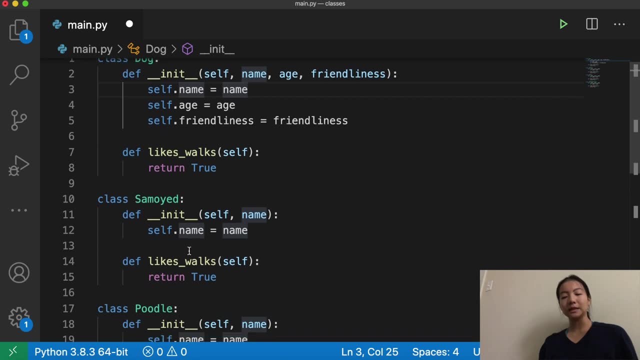 that we have the superclass. remember what we said about how inheritance basically allows the child class to have the same properties as the dog. So we're going to do that And then we're going to inherit from the parent class. all we would have to do is classify our three breeds as child classes. 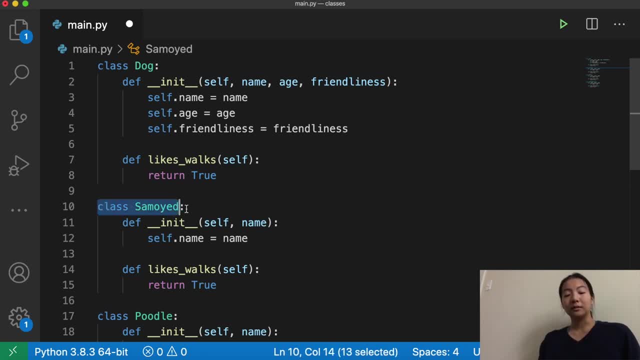 of dog. And how do we do that? Here in our class definition all we have to add is parentheses and then within the parentheses the parent. So here we have Samoyed And then this basically means Samoyed is a child class of dog. And here we can even erase this And of course we would input 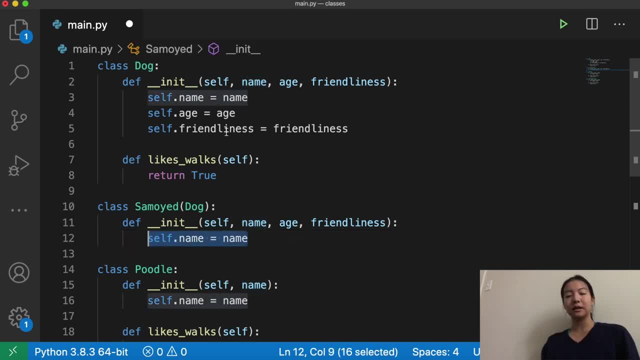 the name, age and friendliness. But then down here, instead of reinitializing the exact same thing, we don't have to copy and paste that code. Instead, we can just do super, And this means called a superclass dot init. So here this is saying in the superclass: called this initialization. 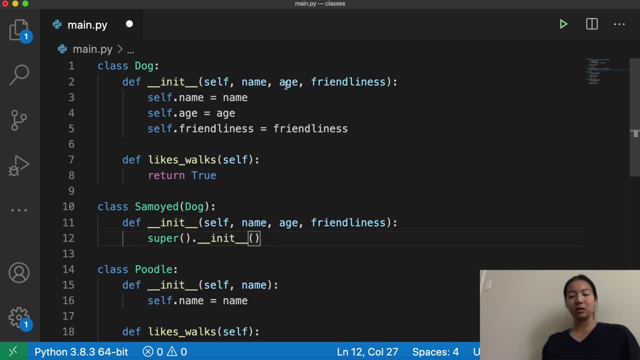 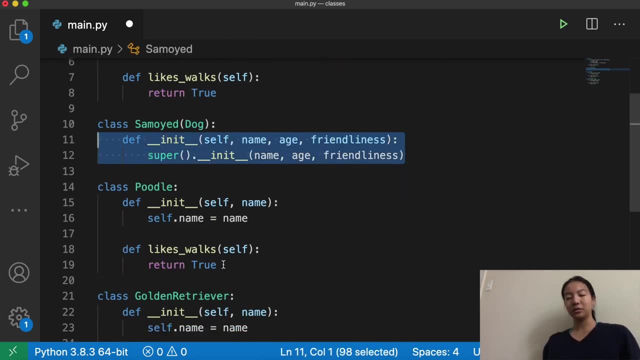 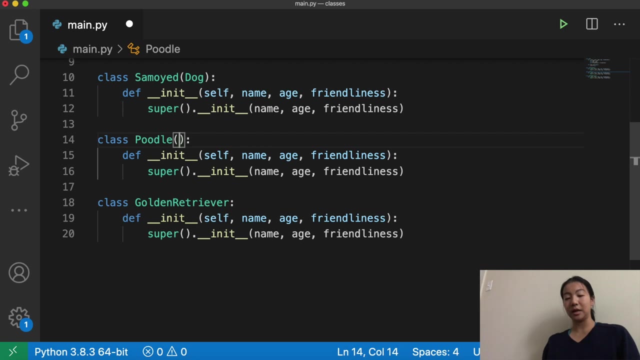 function and then we're going to pass in the parameters that belong up here, So that's name, age and friendliness. And then I'm going to do name, age and friendliness, And then I'm going to do that with all my dog goes down here And change these so that they are now subclasses of dog. 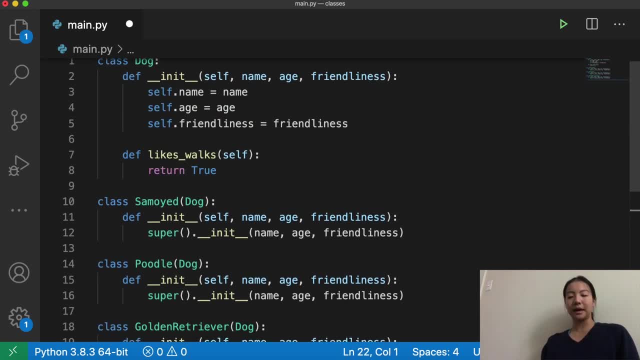 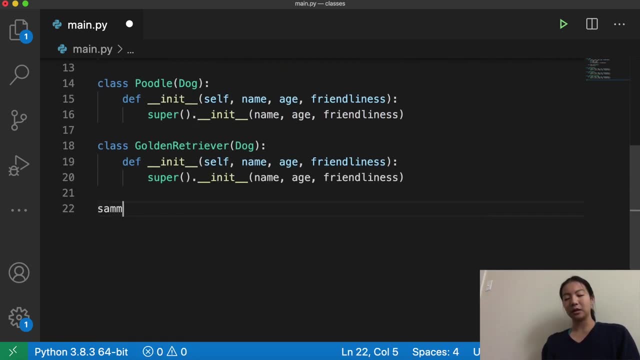 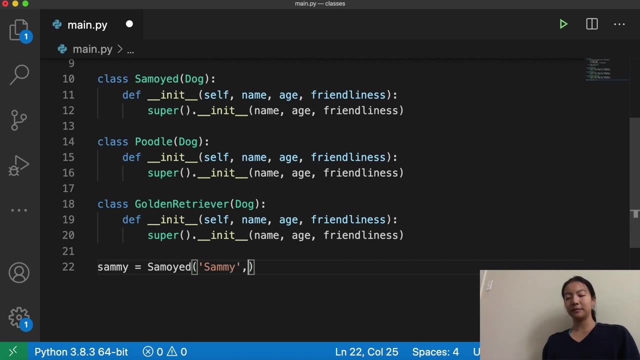 Tada, Alright. so let me just show you guys how this works. You can see that in Samoyed we haven't defined likes walks. But if I create Sammy the Samoyed and I pass in a name, so Sammy, and age to maybe, and then friendliness, let's do a scale one to 10.. Let's say 10.. 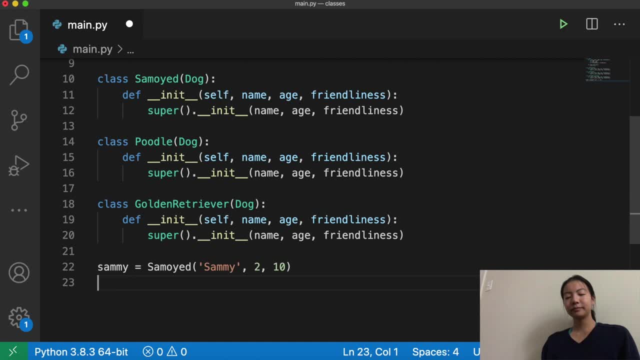 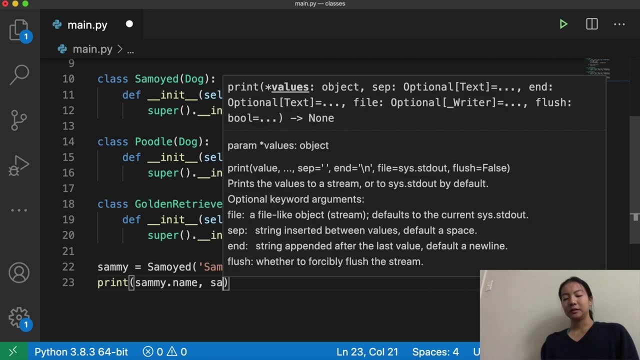 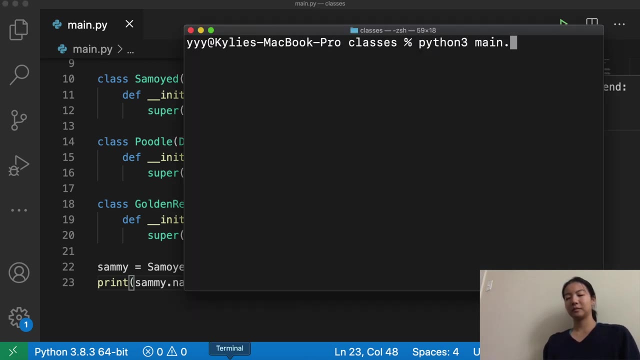 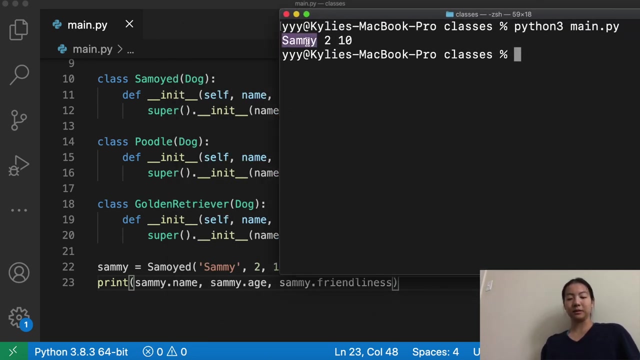 Let's say that Sammy is 10 out of 10 friendly. Okay, so now what we can do is we can print Sammy dot name, Sammy dot age and Sammy dot friendliness. Okay, so we see that for Sammy that the name is Sammy, the age is two and Sammy's friendliness is a 10 out of 10.. So here, 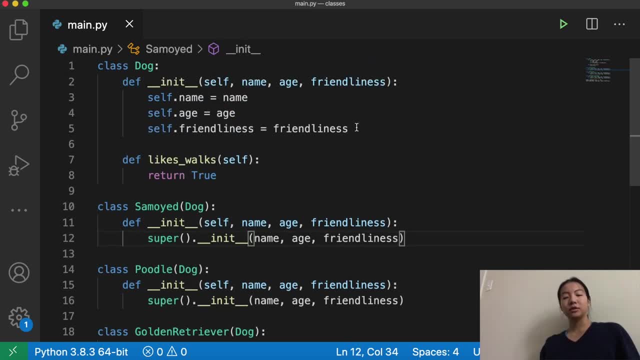 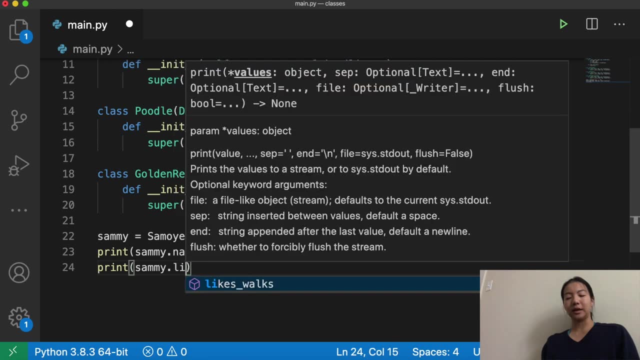 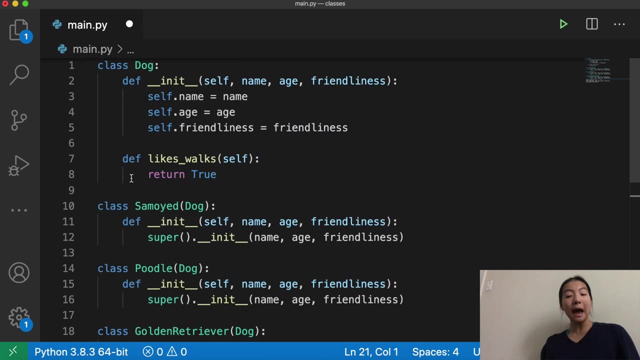 this initialization function has actually called this one up here to set the attributes. Okay. so one other cool thing is we can actually print Sammy dot likes walks. And again, we haven't actually defined likes walks as a method under Samoyed, but we have in the superclass. And now 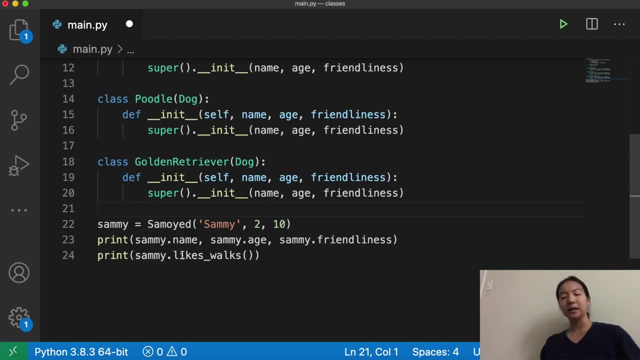 you can see that it will actually inherit Sammy dot likes walks. And now you can see that it will actually inherit Sammy dot likes walks. And now you can see that it will actually inherit from that superclass, So we can actually call this function likes walks. 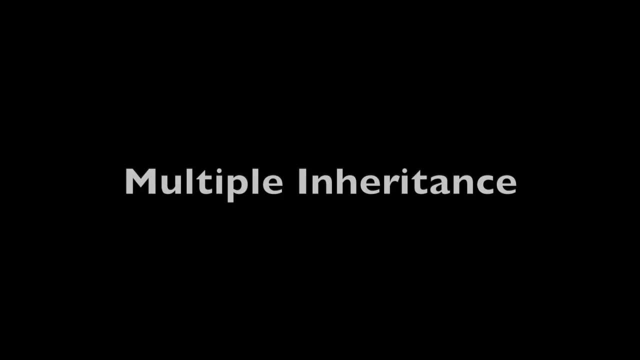 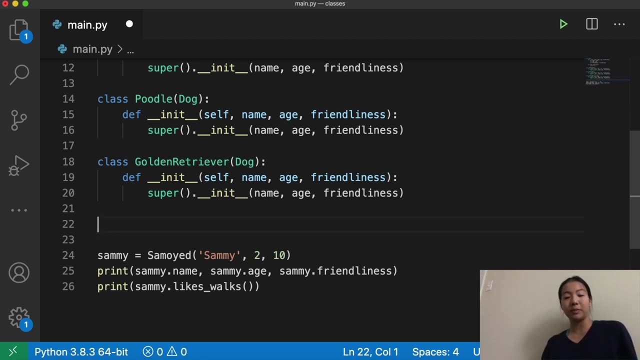 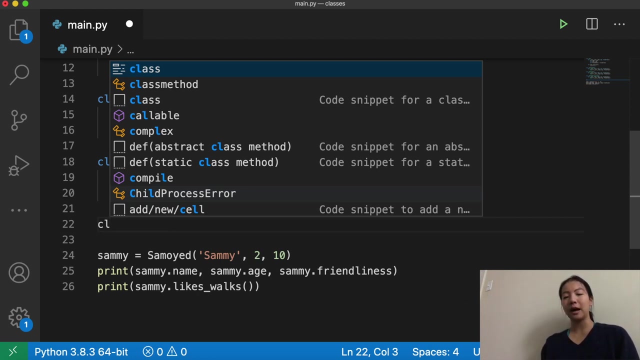 Okay, so look, it's true And, just like in real life, we can also have mixes of these dogs, which would mean that we have more than one parent. So this is something called multiple inheritance, where you can have more than one superclass And the child class would actually inherit all the properties and 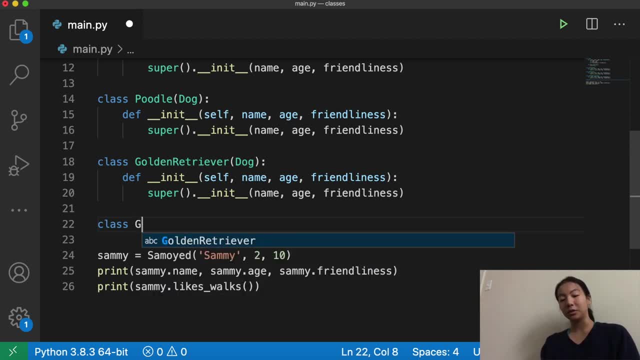 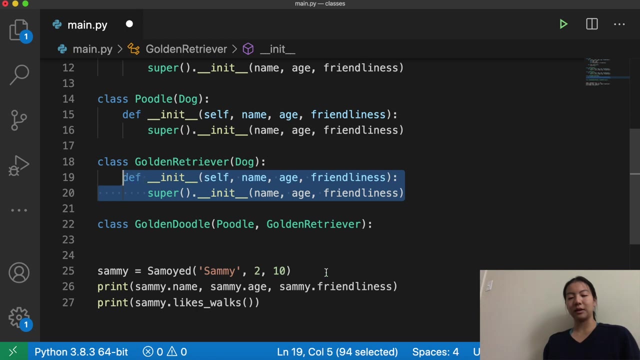 attributes of all the parent classes. So here, if I want to create a golden doodle, maybe, then I can say golden doodle And this is going to inherit from poodle and golden retriever, And of course we initialize this just like how we initialize these other things. 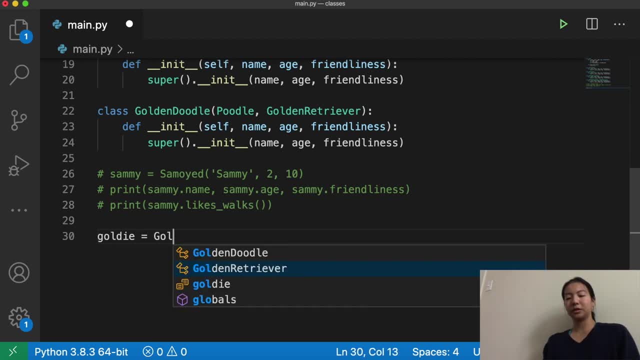 Let's call this golden doodle, Colby, Goldie the golden doodle and Goldie a just do one. We'll mana find that he's 10 out of 10.. And that's how we'll infinite pretzels if we had. 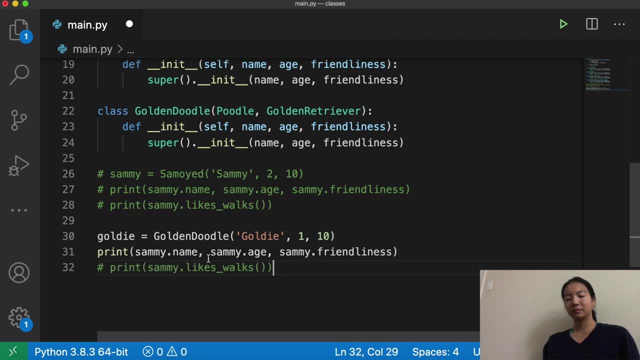 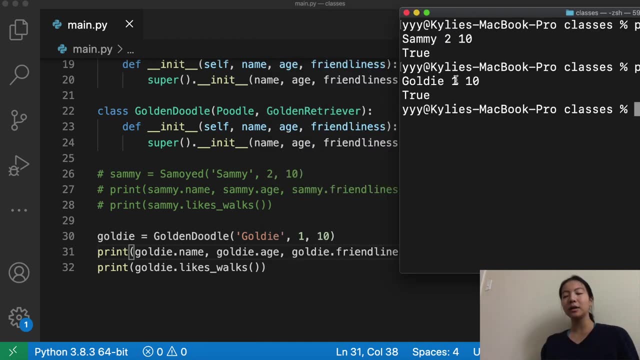 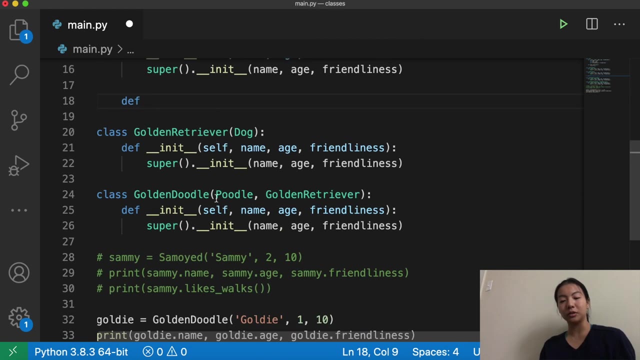 to find the gold in his friend list. we'll be piace incude. thisEN stood for next. So we like Klein Goldie, golden retriever Here. if I want to differentiate this, let's say tastes that were different where Goldie was 18.. And then I can also. 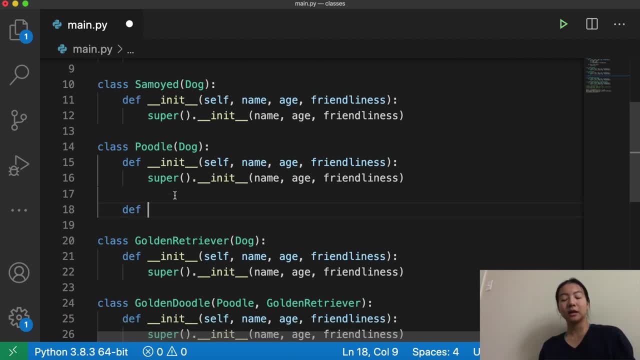 print this one, So endurance 10,. you could print golden. I can print Obsidian and like know goldie And in these inspire myself 18.. So if I need one of these friends here, I can just look on this. Also, if I have different swaps, I can print goldie. golden retriever, which is 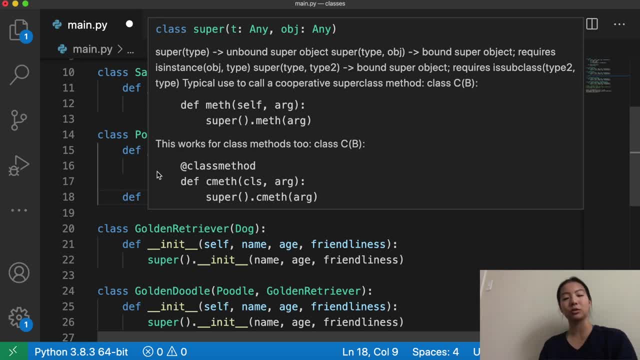 very similar to my friend list. So they're just buying Golden doodle呼: GDP 10, odds over 10.. So I can go here that the one class We're getting the Goldie Gold from Goldie, a Golden property that we actually want to pass down into this golden doodle. 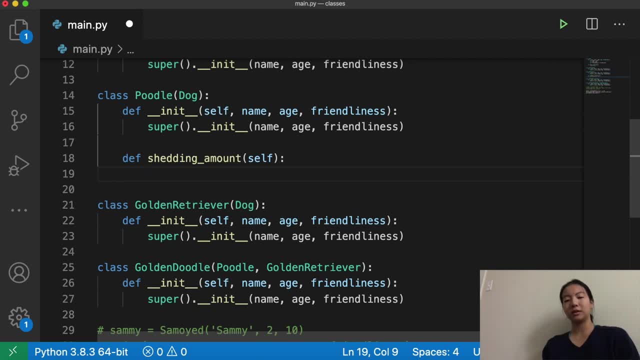 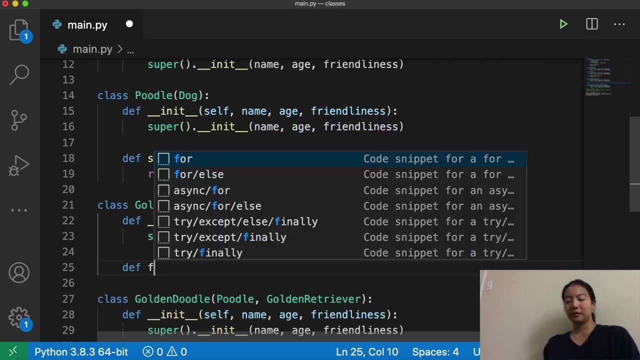 So, for example, our shedding amount. well, poodles don't shed, So here we're going to return zero. And then for golden retriever, let's do one. that's like define fetch ability, And this is a method. 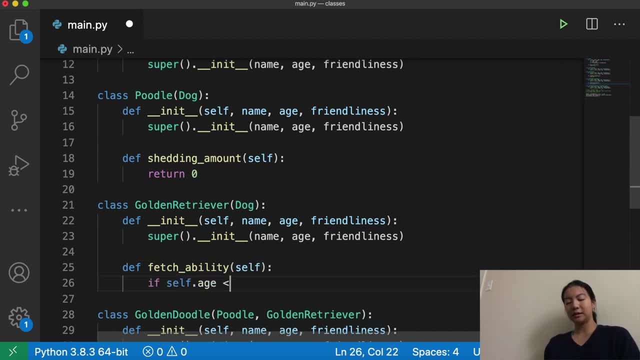 So let's say the soft dot age is less than two. maybe the golden retriever is not that great at fetching yet, So we'll give it an eight out of 10.. So return eight. But let's say else if the age is less than 10.. 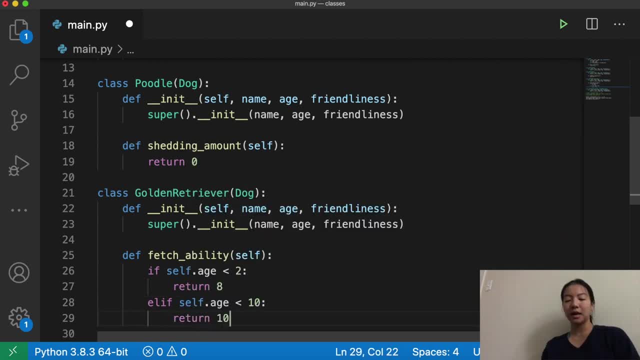 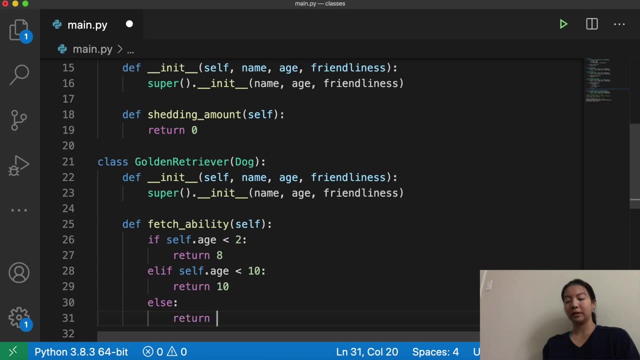 So this is maybe something between two and 10.. We can return 10 out of 10. And then otherwise, which means that it would actually be older than 10.. We can return seven, because maybe they're a little bit slow. I don't really know. 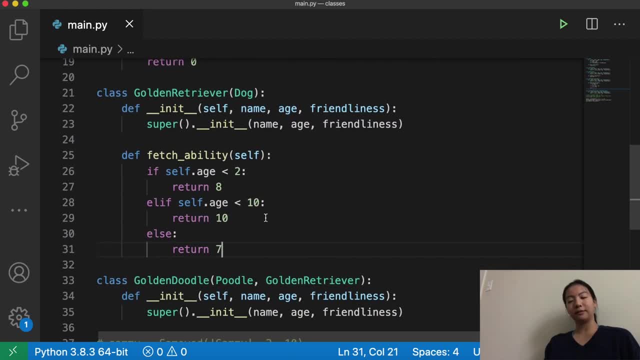 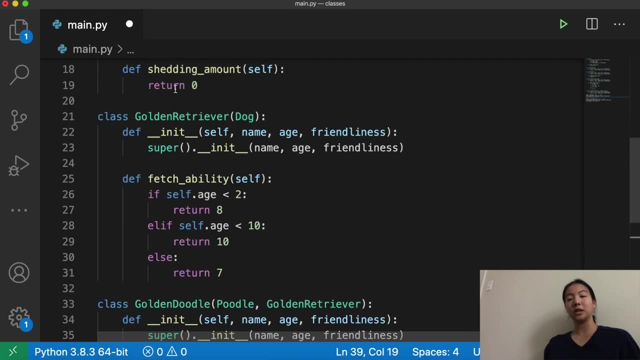 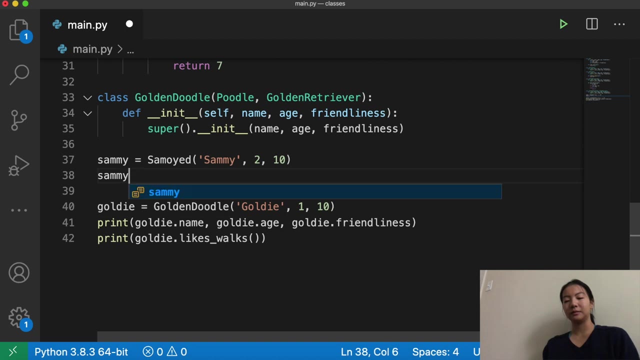 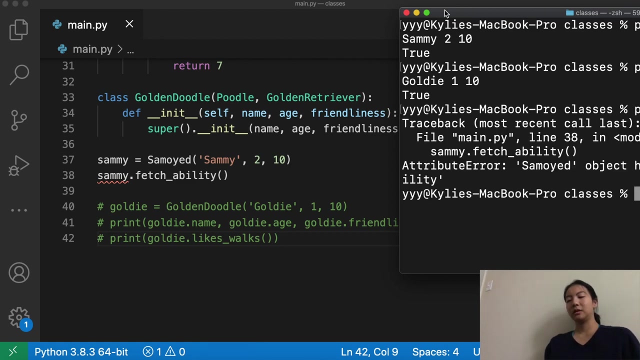 So here let's try Sammy. can Sammy fetch? Well, we haven't defined this fetch ability function under Samoyeds And it's not defined under the superclass dogs. So when I call Sammy dot fetch ability, it would actually come out to an error, because 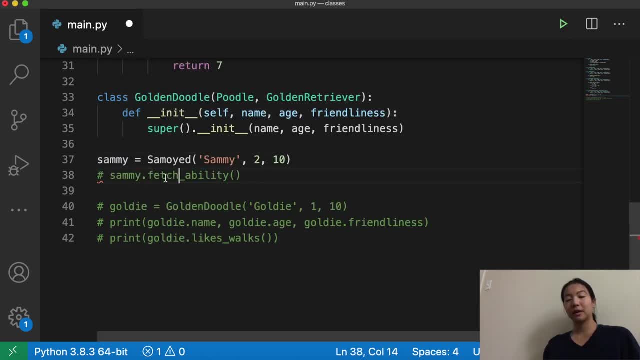 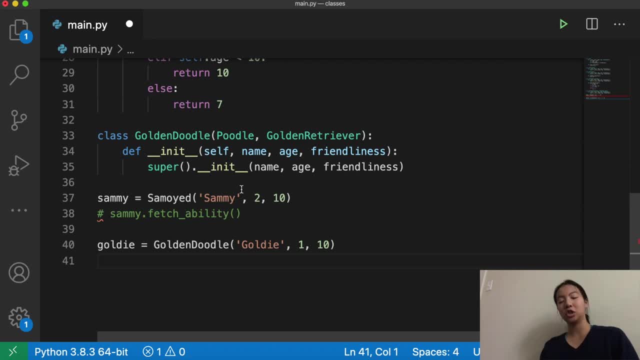 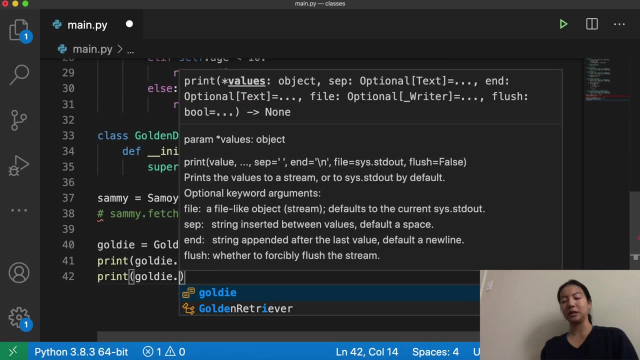 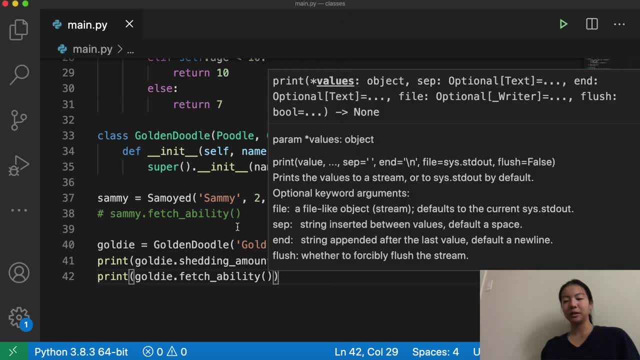 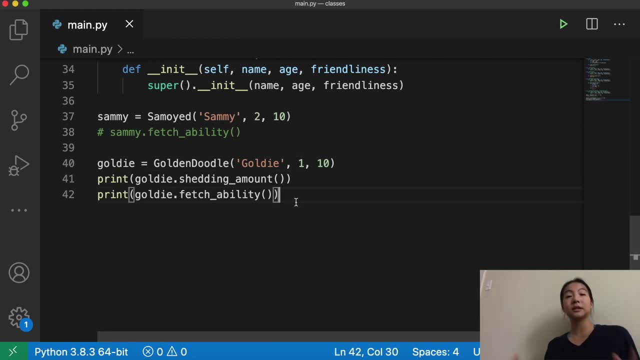 And here we get a shedding amount of zero and a fetch ability of eight, because Goldie is less than two years old. Ta da, Okay. so just to quickly sum things up a little bit: inheritance means that you have children classes that can actually inherit properties from parent classes, and then multiple inheritance means that you 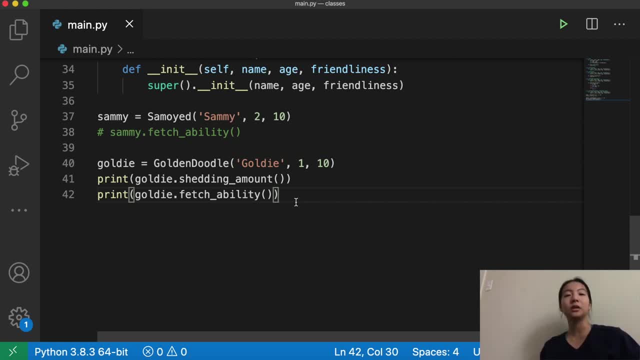 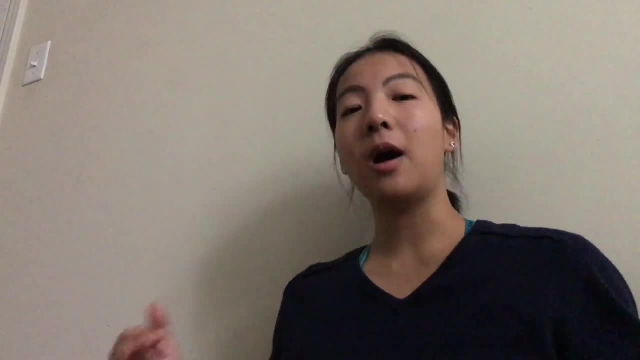 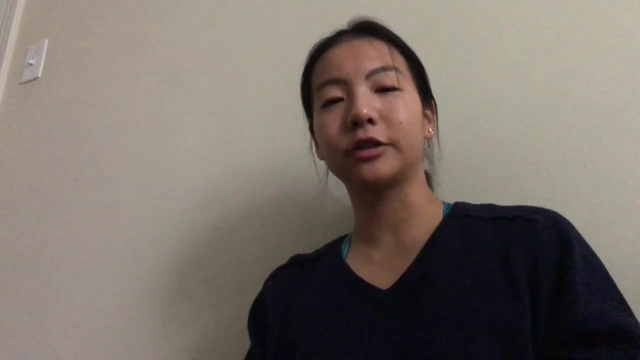 can actually have more than one parent, where the subclass will inherit from all of the parents. Okay, so let's talk a little bit about Holly morphism. now, what in the world does polymorphism means? Polymorphism Quite literally means the ability to take multiple forms from an object oriented. 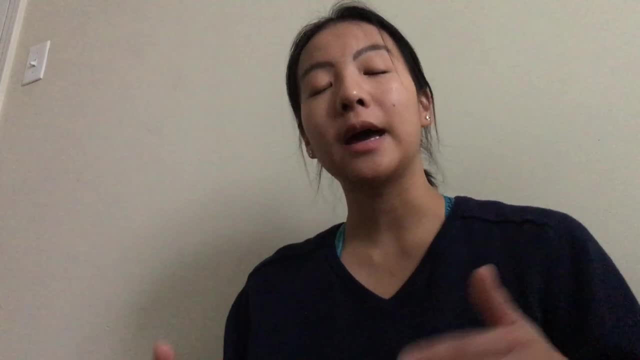 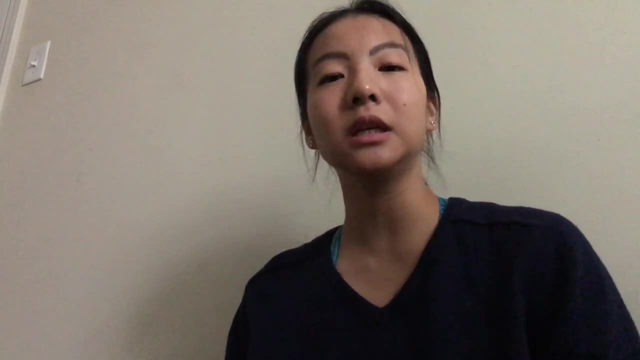 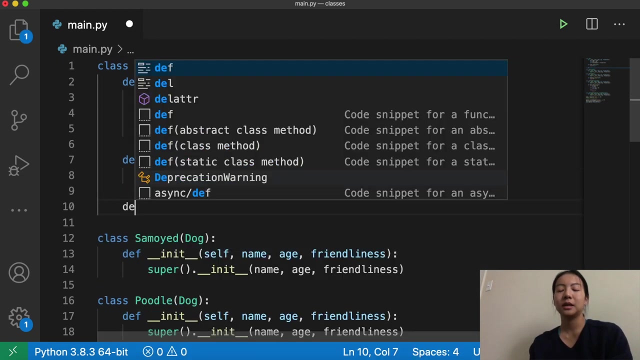 standpoint, This actually means that a child class that inherits a function from maybe the parent class can override that function and give that function a completely new set of rules to follow. So again, let's do an example with our dogs. under our dog maybe we can define our bark. all dogs might bark like wolf, So we can return. 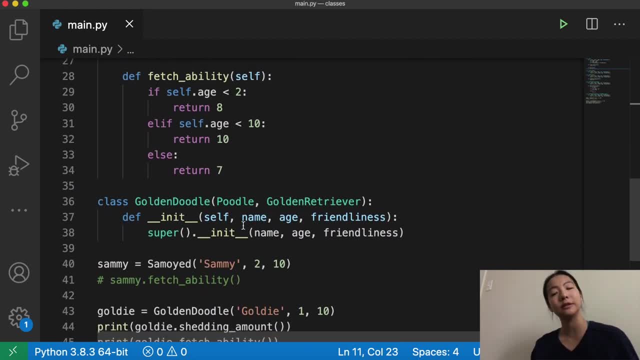 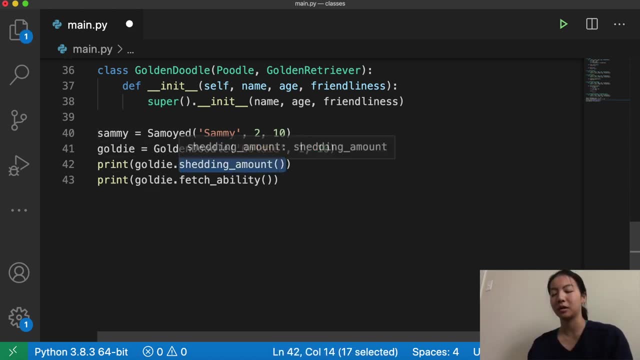 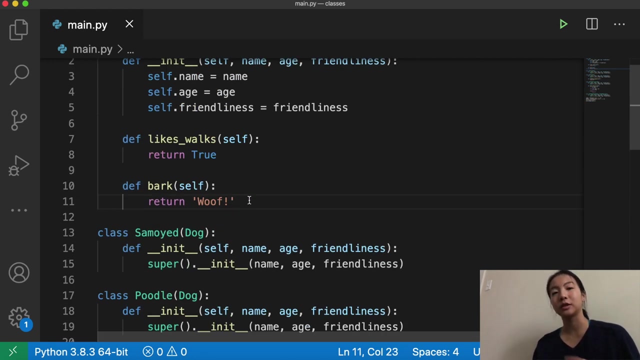 wolf as our bark for all of our dogs, And that's just our default bark. Okay, so we have Sammy and we have Goldie. Let's just see what their bark would sound like. Okay, so we're printing Goldie's bark and Sammy's bark And both of them are wolf, But we can actually change this for subclasses.